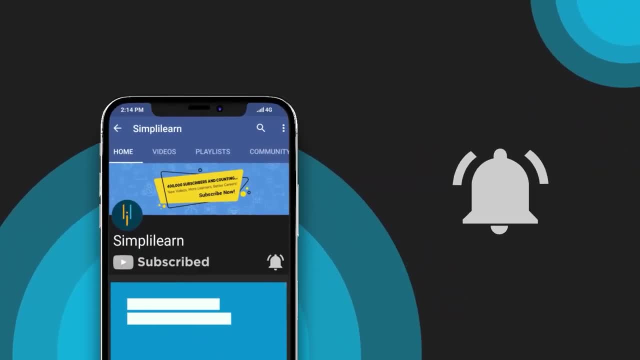 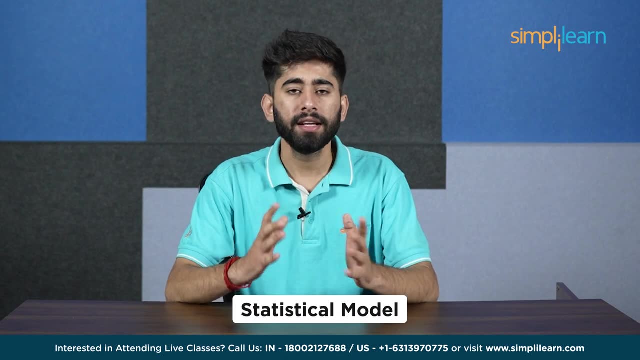 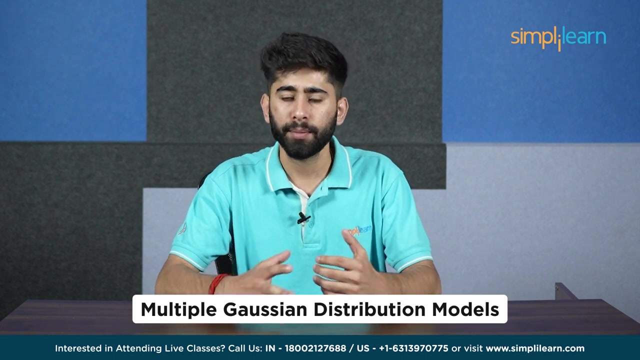 A Gaussian mixture model, also known as GMM, is a statistical model used to describe data distribution. It assumes that the data can be represented as a combination of multiple Gaussian distributed models, each with its own mean and variance. In practice, this means that 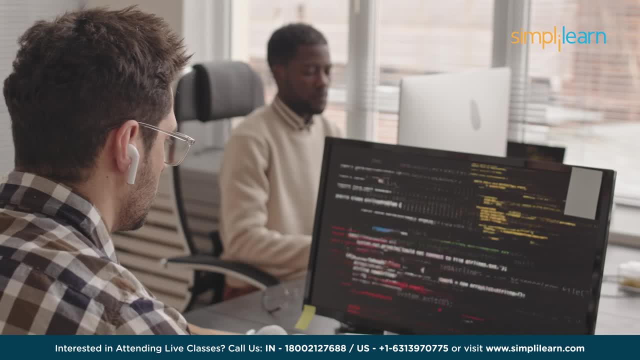 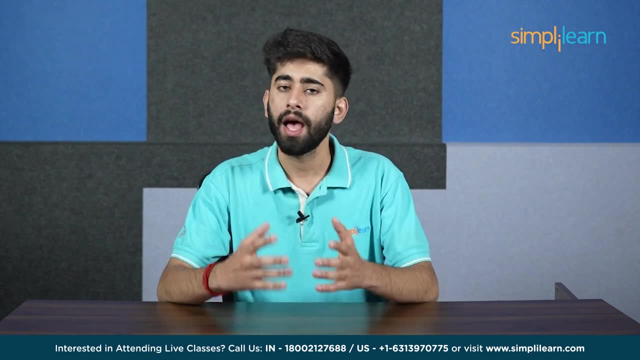 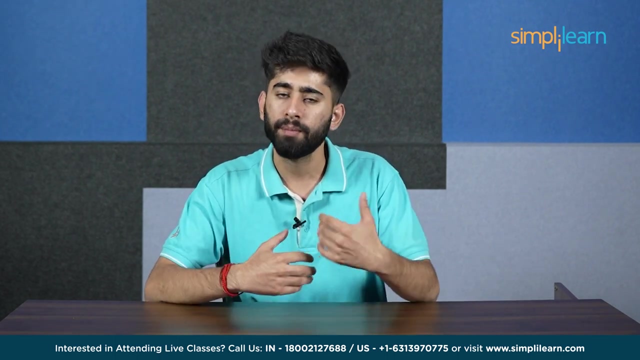 we can model complex distributions, such as the distribution of test scores or income, by combining multiple simple distributions, such as distribution of a test score of girls and for boys. Using GMM to model a distribution allows us to capture the complexity of the data and describe it more. 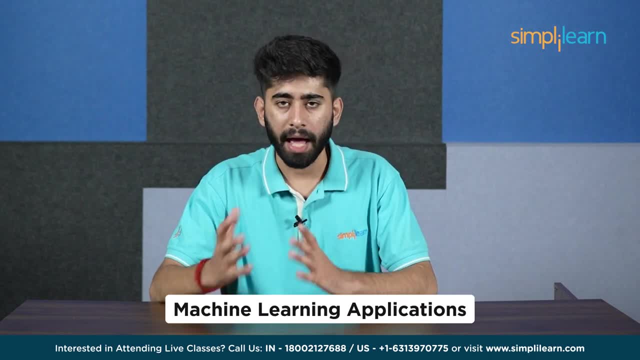 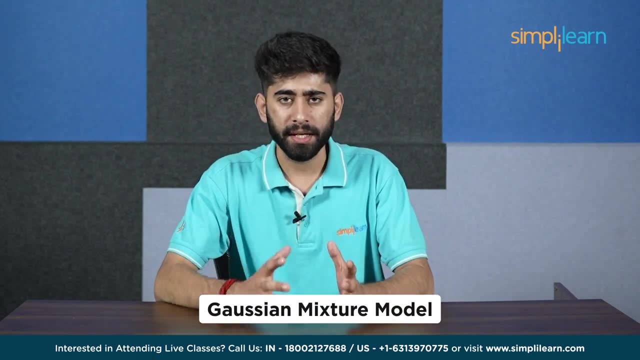 accurately. This can be particularly used in machine learning application, where we often deal with complex and high dimensional data sets. Let's now deeply understand the Gaussian mixture model and Gaussian mixture distribution. So, without any further ado, let's jump on to our topic. 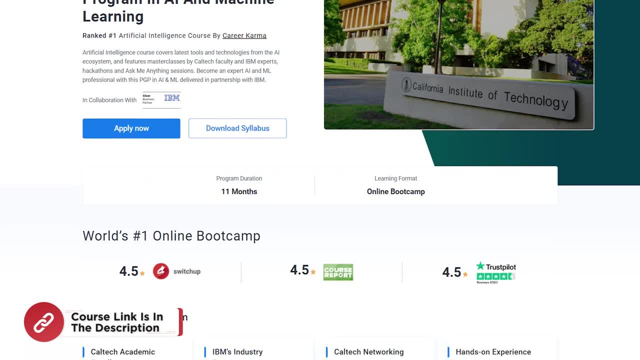 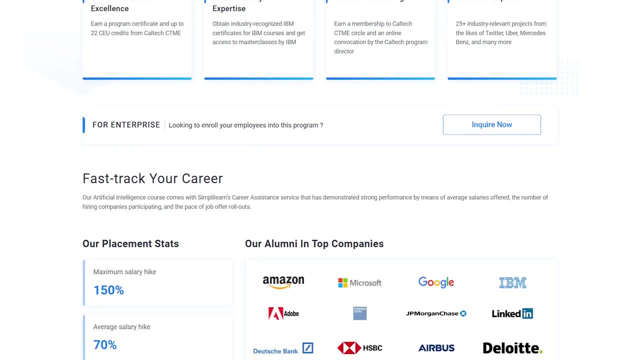 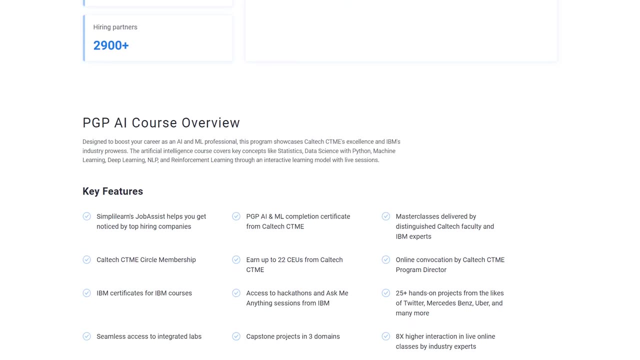 In this rapidly expanding field, you need to develop the right skill. if you want to boost your career in the field of ML, Then take up our Caltech postgraduate program in AI and ML partnership with IBM. that will help you become an expert in AI and ML. This course covers the latest tools and technologies and features. 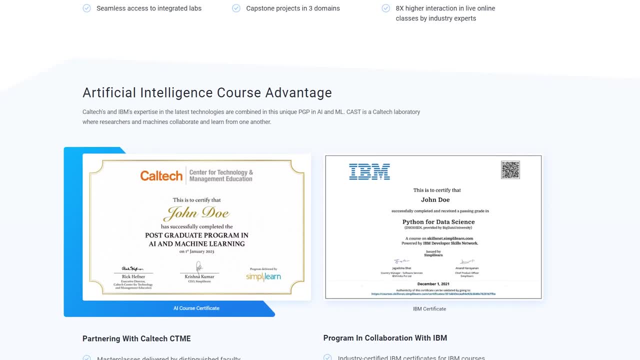 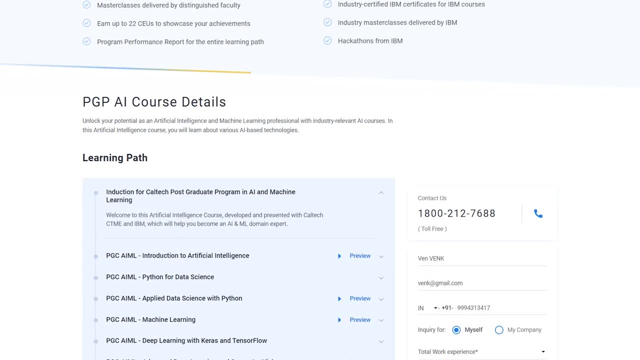 masterclasses by Caltech faculty and IBM experts. Hackathon and ask me session are also there. These are a few reasons you should take up this course. If you are interested in learning more about AI and ML, please subscribe to our channel. You should consider learning machine learning Now. enroll in Caltech postgraduate program in AI and 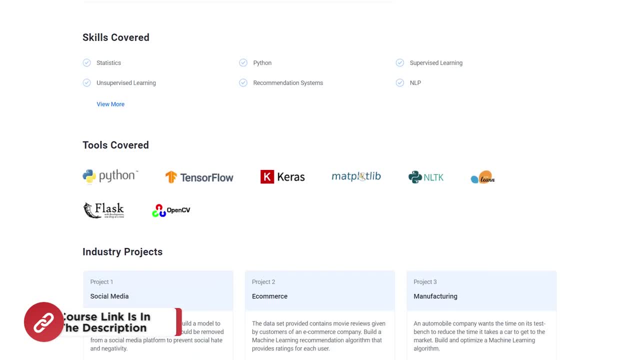 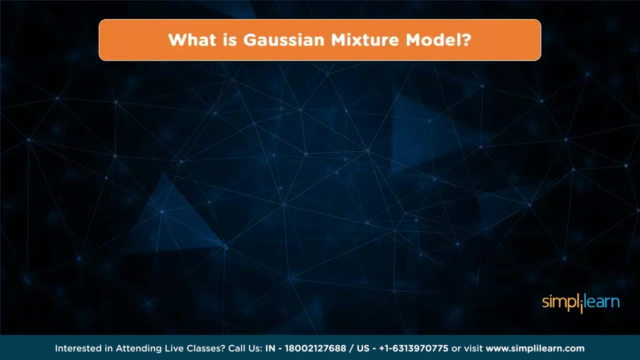 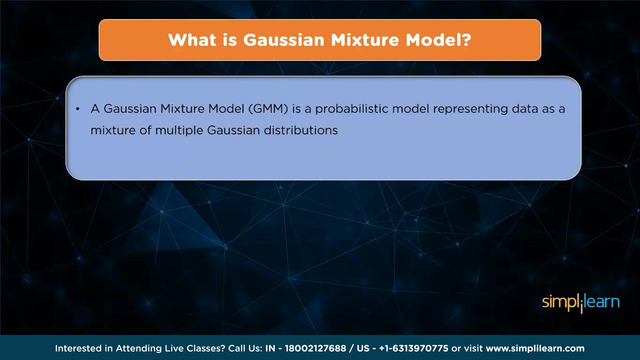 ML and become an ML engineer. The link will be in the description and pinned comment. Now let's start this video and see what is Gaussian mixture model. A Gaussian mixture model is a probabilistic model representing data as a mixture of multiple Gaussian distributions. 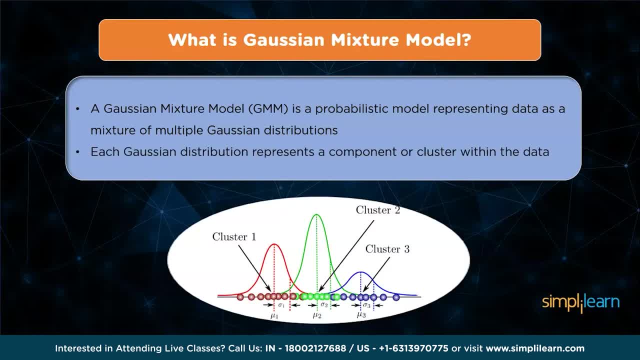 It is a mixture model because it assumes that data points are generated from a mix of Gaussian distributions, each associated with a certain probability In GMM. each Gaussian distribution represents a component or cluster within the data. The model assumes that the data points within each cluster are generated from a Gaussian 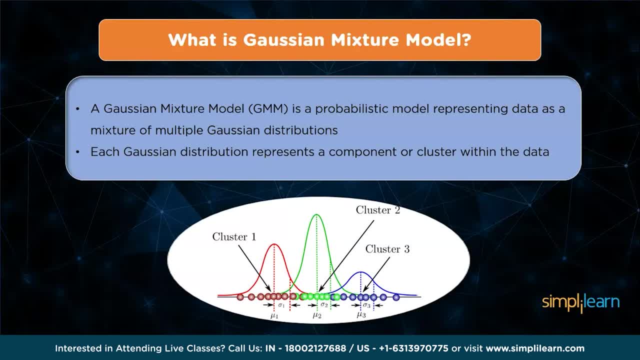 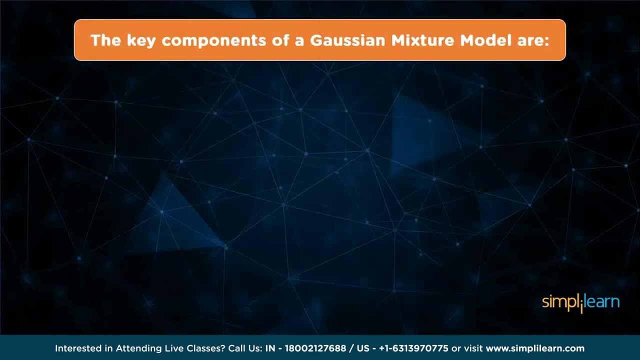 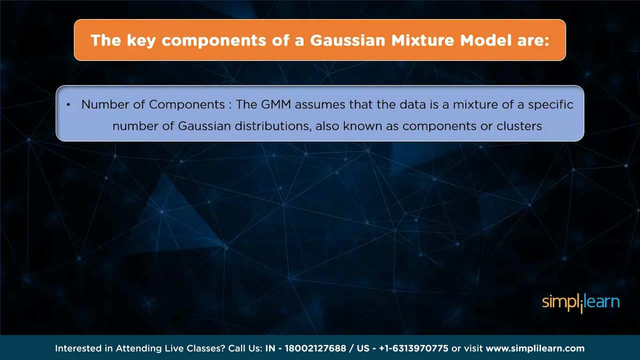 distribution with its mean and covariance. The GMM, which is known as Gaussian mixture model, combines these component distributions with mixture weight to form the overall probability distribution of the data. So now let's see the key components of Gaussian mixture model. So the number one is number of components, also known as clusters. The GMM assumes that the data 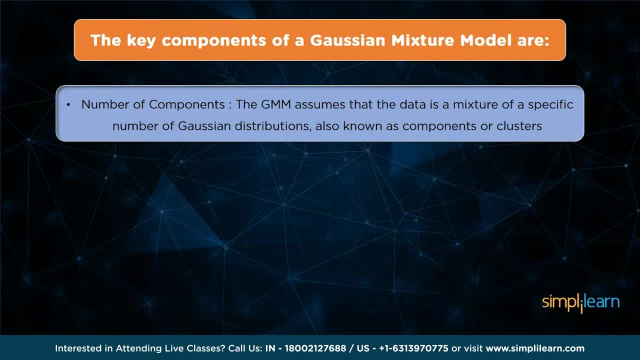 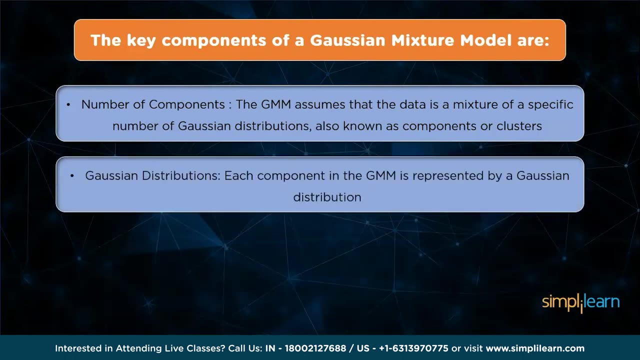 is a mixture of specific number of Gaussian distributions, also known as components or clusters. The number of components is typically determined in advance or estimated by using techniques such as model selection. Next, we have Gaussian distribution. Each component in the GMM is represented by a Gaussian distribution. A Gaussian distribution. 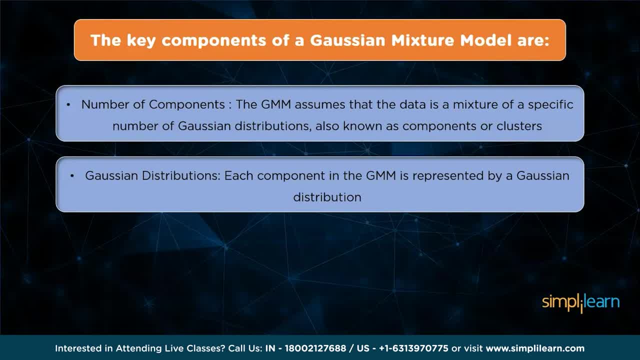 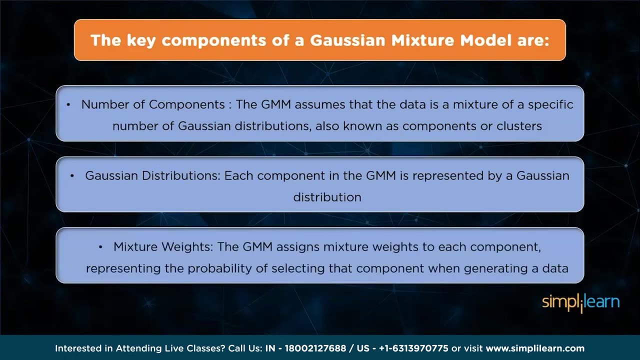 also known as normal distribution, is a bell shaped curve fully described by its mean and covariance. The mean represents the center of the distribution and the covariance determines the spread or shape. The third one is Mixture weight. GMM assigns Mixture weight to each component representing 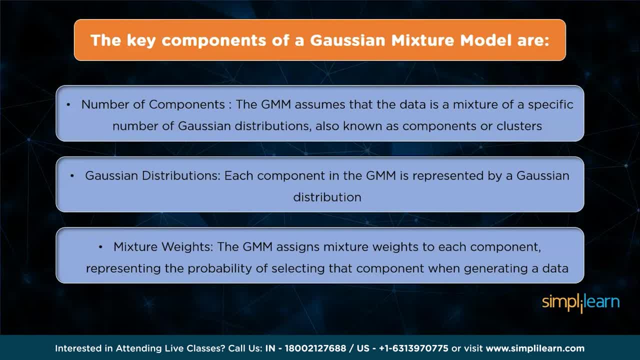 the probability of the distribution. The GMM also assumes that each component of GMM is a mixture of of selecting that component when generating a data point, These weights must sum up to one. The mixture weight determines the collaboration of each component to the overall distribution. 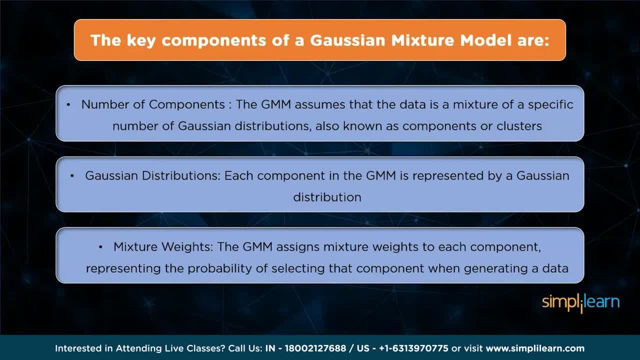 So by using a Gaussian mixture model, involves estimating the model parameters, including the means, covariance and mixture weights. This is typically done through an interactive optimization algorithm. like the exceptional maximization algorithm, The EM algorithm alternates between the estimating the responsibilities of each component for each data point. 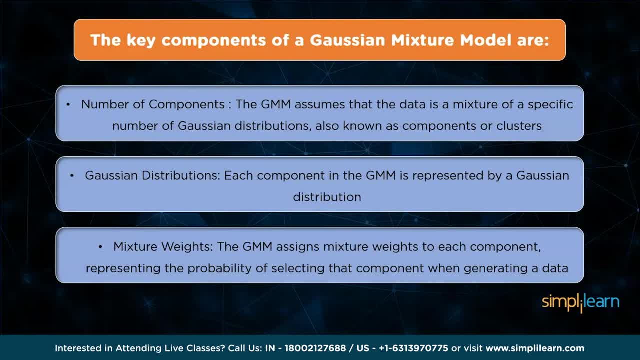 and updating the model parameters based on the responsibilities. The algorithm continues until convergence, where the parameters reach a stable state. Once the G is trained, it can be used for various tasks. For example, it can be applied to clustering by assigning data points to the most likely component or cluster. 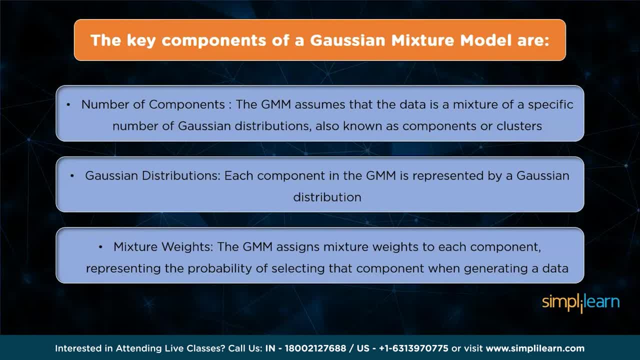 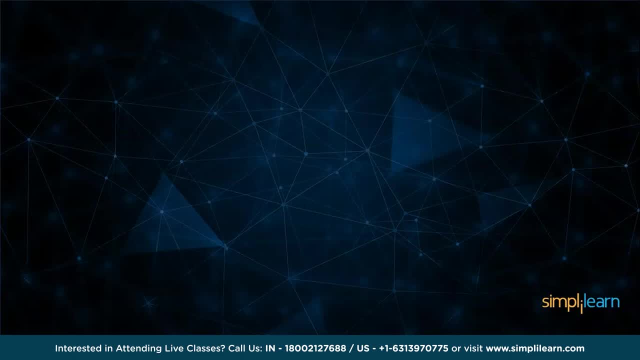 It can also be used for density estimation. Variety of data points can be applied to the most likely component or cluster. Variety of data points can be applied to the most likely component or cluster. It estimates the underlying probability distribution of the data. Now let's see what are some real-world examples where Gaussian mixture model can be used. 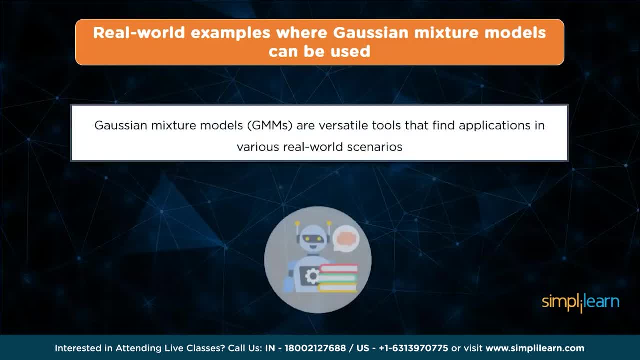 Gaussian mixture model, also known as GMMS, are versatile tools that find application in various real-world scenarios. They are particularly useful when dealing with large datasets, where identifying clusters is challenging. GMMS excel at efficiently discovering clusters of Gaussian outperforming clustering algorithms like K-means. 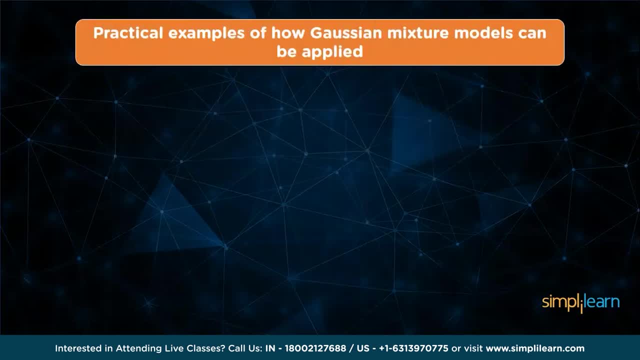 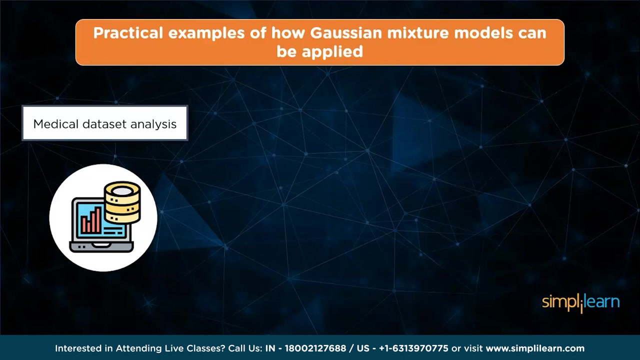 Now here are some practical examples of how Gaussian mixture model can be applied. The first one is medical dataset analysis. Gaussian mixture model can segment medical images or identify patterns within metasets. By clustering patients based on similar symptoms, GMMS can assist in detecting diseases, subtypes, predicting outcomes and reliving questions. 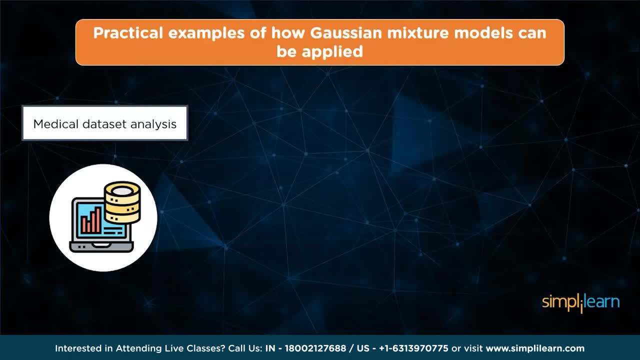 And revealing previously unknown patterns in large-scale patient records. Next, we have modeling natural phenomena. GMMS are suitable for modeling natural phenomena where Gaussian distributions are observed in the noise. This modeling approach assumes an underlining unobserved entities or attributes, with measurements taken at central point across multiple observation sessions. 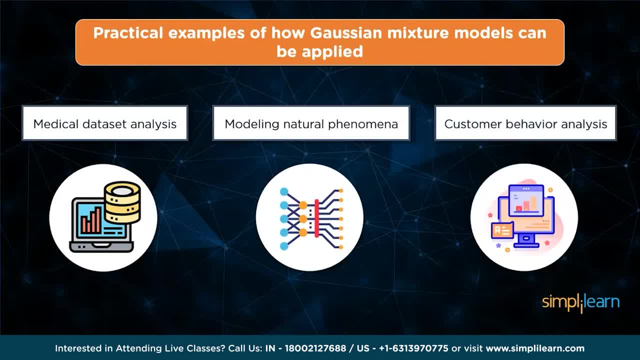 Next, we have customer behavior analysis. Gaussian mixture models are valuable in marketing for analyzing customer behavior. By leveraging historical data, GMMS can predict future purchases, enabling businesses to tailor their market strategies and get more efficiently. Next one is stock price prediction. 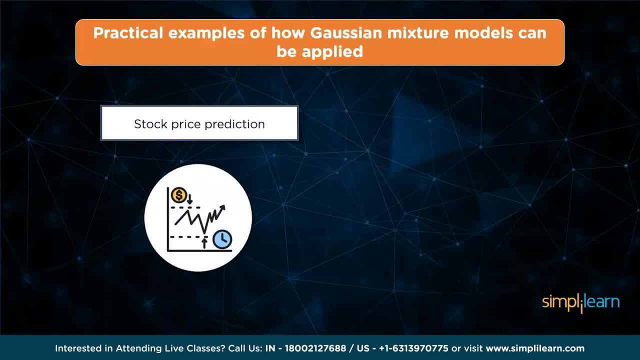 Gaussian mixture models find applications in finance, especially in analyzing stock price time series. They can identify challenge points within the data, helping detect turning point in stock price or other market movements that might be obstacled by volubility and noise. Next we have gene expression data analysis. 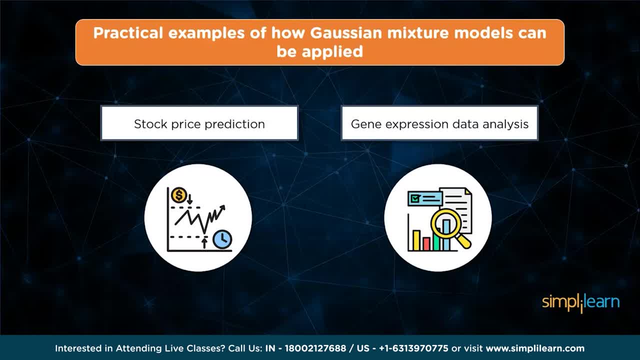 Gaussian mixture models are employed in gene expression data analysis. They can be utilized to identify differentially expressed genes between two conditions and determine which genes may be due to specific phenomenon type or disease states. Now let's see the implementation of the Gaussian mixture model. 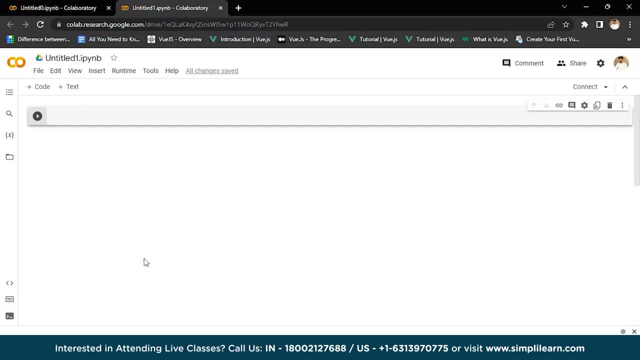 Now to do this small demo. I have taken an iris dataset. Okay, In Python there is a Gaussian mixture class to implement GMM. Load that iris dataset and then we are good to go. First thing we're going to import is our numpy, which is a library of Python. 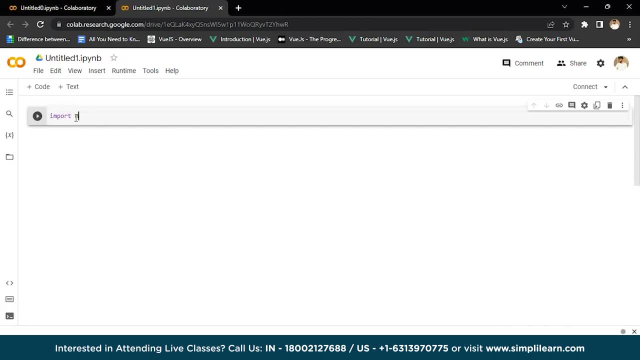 Okay, so we'll write import numpy as np. In the next line we have to import panda, So we'll write import panda as pd, And after that we'll import matplotlib, We'll write import matplotlibpylo. We'll also write import pdt as dlt. 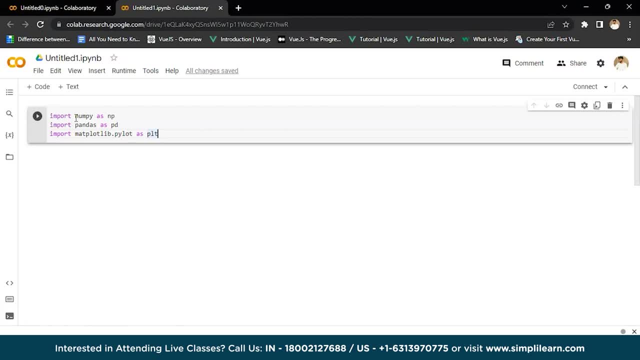 Okay, till then I guess it's fine for us. Yeah, So now we will write. from pandas: we will import data frame. Okay. After that From scikit-learn, which is SKLearn. sklearn will write it will. from sklearn will import dataset. okay, and then again from sklearn. 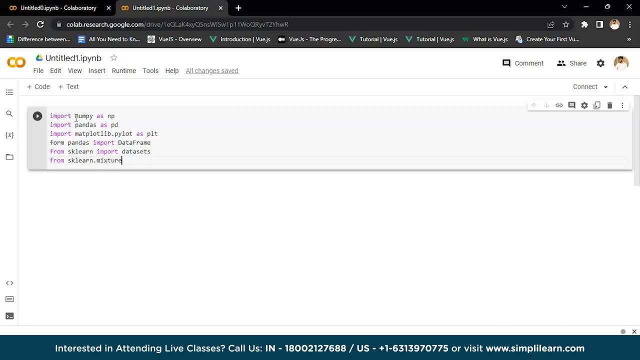 dot mixture will import gas in mixture. now we'll load the irish data set. for that we'll write irish the name and then data set that we just now imported from sklearn. we'll write data sets- dot load, because we need to load that data, and we'll write this, this function sign. after that we'll give it a variable x and 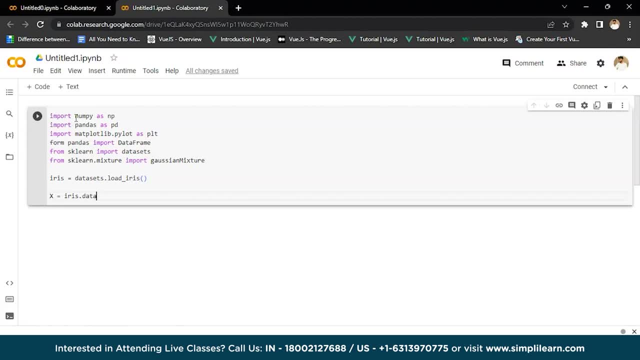 irish dot data from. so the semicolon we just wrote is for everything, like all the data. when we have to show all the data, we'll write this: imagine there is a array of seven uh things, zero, one, two, three, four, five, six, okay, and you want everything of that array, so we'll use this keyword. 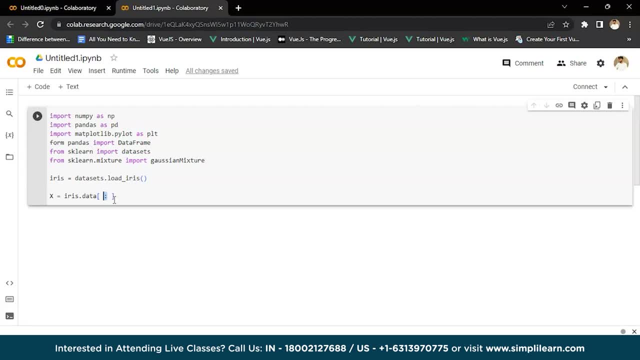 want only, out of that, seven. if you want only five, so we'll write here comma and then we'll write two. so what it? this will show us only five: zero, one, two, three, four. okay, yeah, now we will write d, which is pd dot data frame. you will see, we'll get the data frame from x. 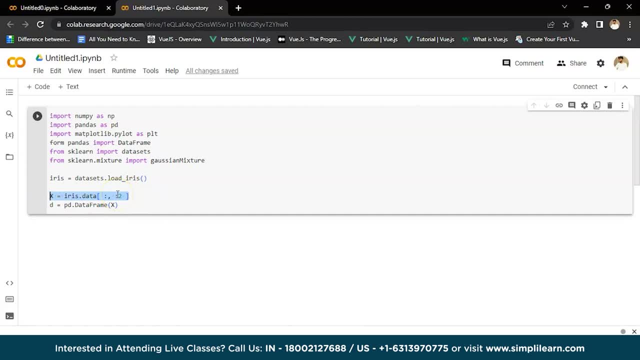 that we just declare. so this is for the turn into a data frame, for, like, turning into my data into a data frame. okay, now we have to plot the data. for that we'll write plot dot scatter and then we'll write d of zero of one right, and then we'll say: 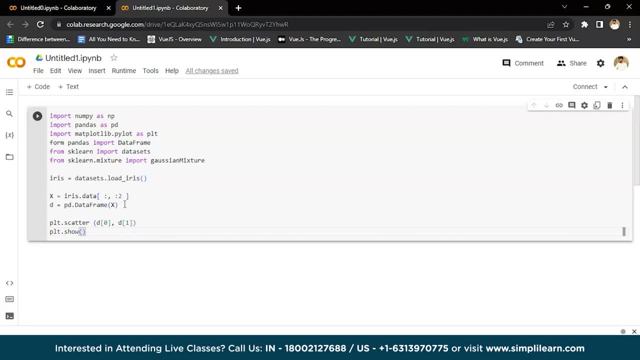 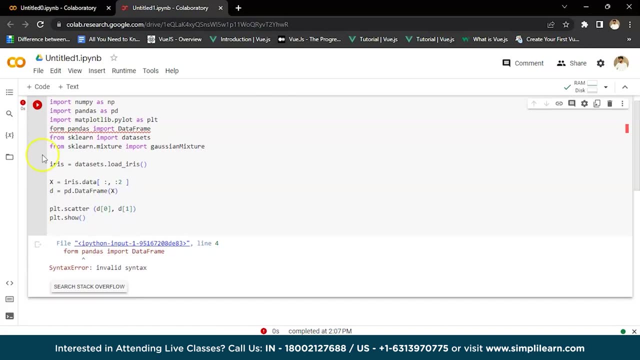 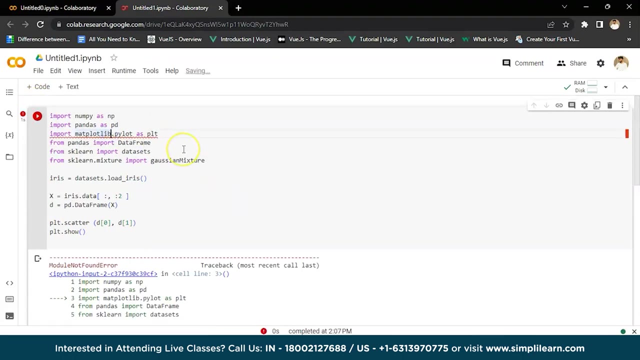 show, and now let's see if it works or not. okay, it's showing me one error, so let's see. okay, got it, that's my mistake. now let's run it again. it's showing my plot lib error again. let's see if i am not many spelling mistakes here. okay, let's give it a chance again. 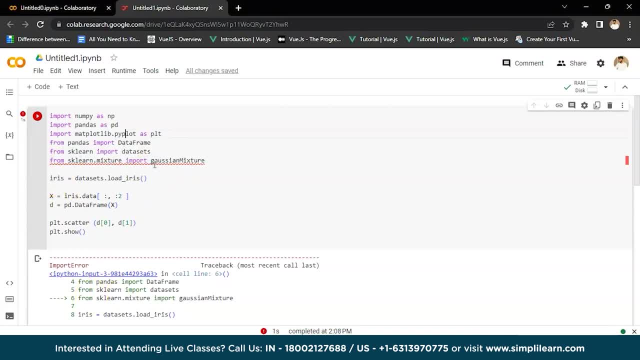 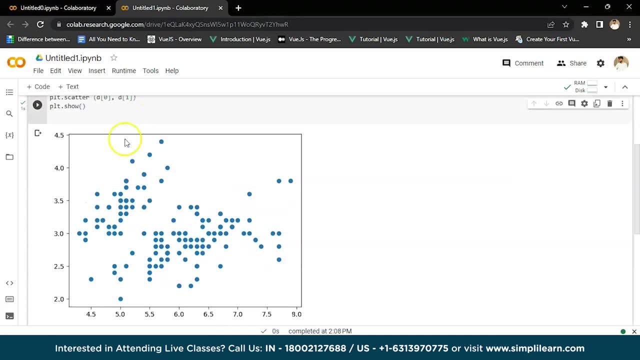 can. some error is there? oh yeah, gas and mixture should be in capital. everything looks fine this time. yeah, so you can see the data. now. you will see the data of these flowers, irish flowers. it's like everything is mixed. you can identify which one is which and you can identify the exact. 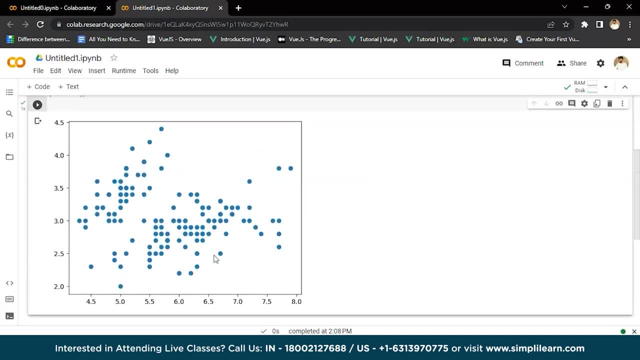 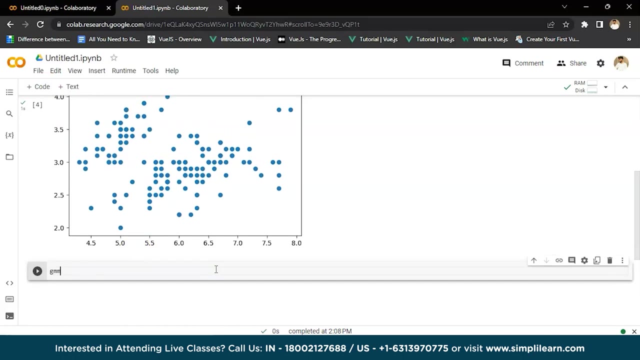 things that you want to see in this data. so for that, cation mixture comes in. so with this method we'll see the difference between the things that we want to see in the data. okay, so we'll click on the plus sign and we'll write mm. glassing mixture model equals to sign and gasion it's showing us. 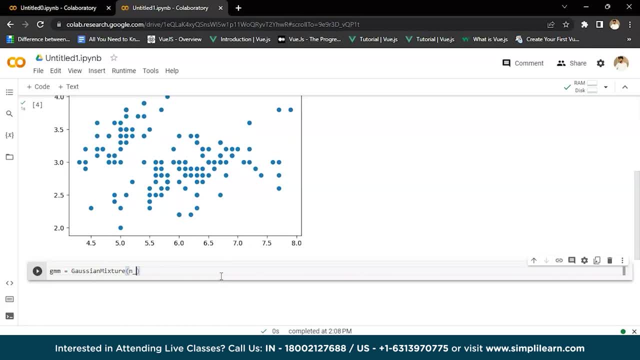 and and two components equals to three. yeah, so we'll keep going find the gmm model for the this data set and with the three gaussian distribution so that we can see the different colors for every data set in this. so we'll give gmm dot fit and the data frame. 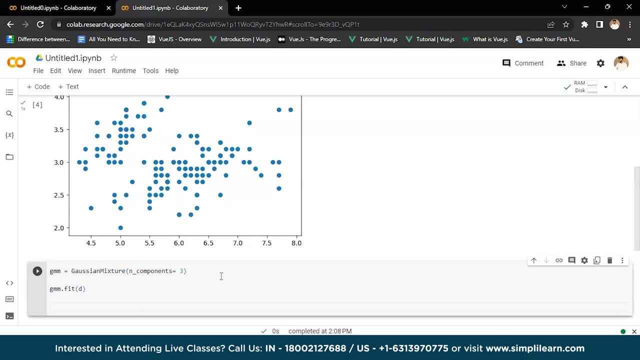 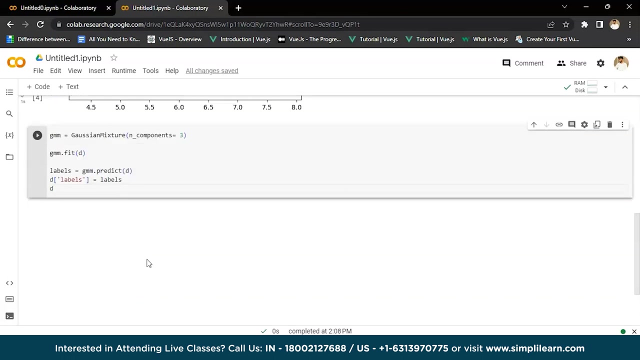 of the data and now we'll just assign a label to each sample. okay, for that we'll write label equals to gmm. dot. predict the data data. now we'll give this data a label that will write the label: labels equals label. okay, and and write d0 and we will give this d0 label so that we can identify it later at which one is. 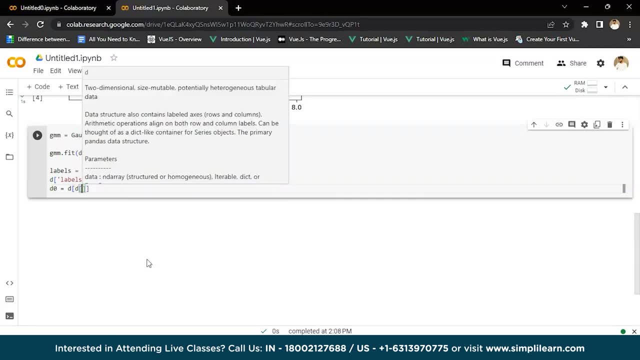 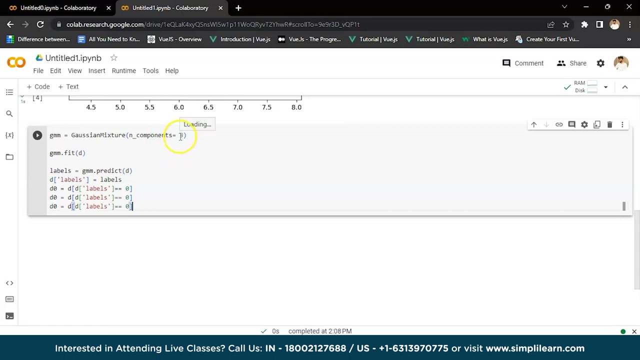 the data of ours. okay, so we'll again write labels. equals to zero. okay, this one is for zero and we'll copy this and we'll paste it three times. yeah, so, because we have taken the components three. if it's more, we can use more also. so we have to change the value of d1- d2. 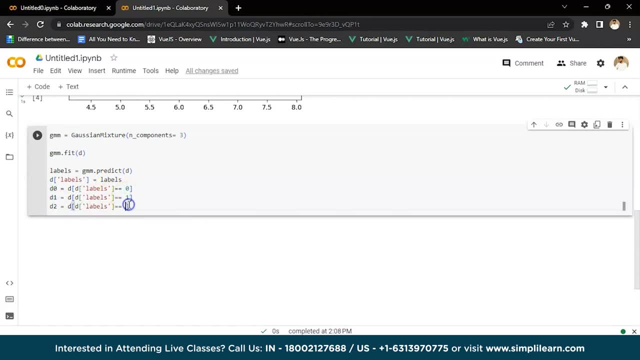 and here also we have to change the values or the output will be not come like what we want the output to be. okay. till now we have assigned the label. okay, now we'll move forward. we'll plot three clusters in same block, okay, so for that we'll. 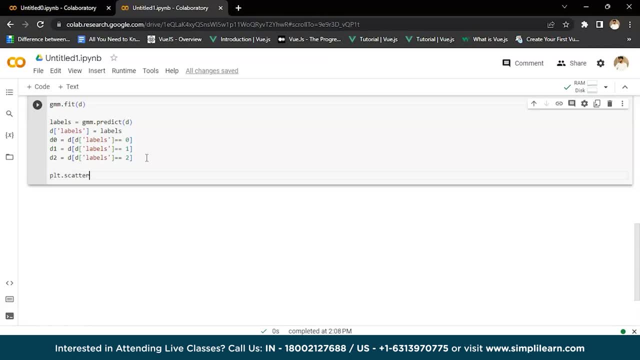 write plot dot scatter from d0 to comma d0 and then one, and we will make this as red. we have to write this in the column, lire in the column. so the color should be relatively linear from here. so the color should be qualitative in Whatever others can say. 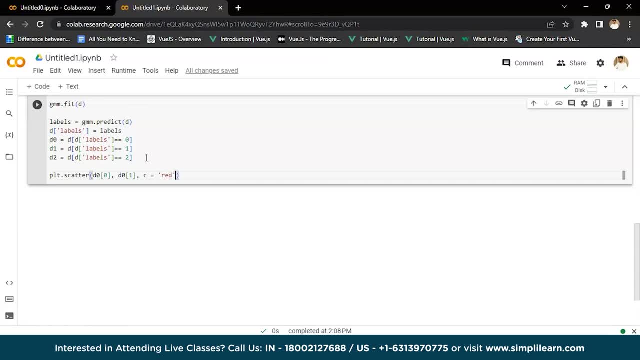 one, two, three goes. that was previously given. one, two, three, four. and if you will do the same thing烈 Re, then it will go ahead. let's put some layer into every corner, red in the column, so the color should be shown on the screen. okay, so we can just copy this line. 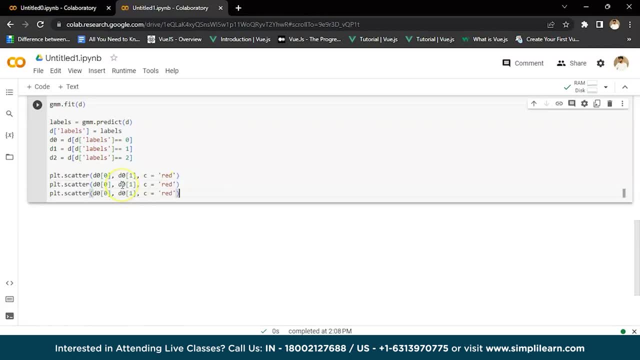 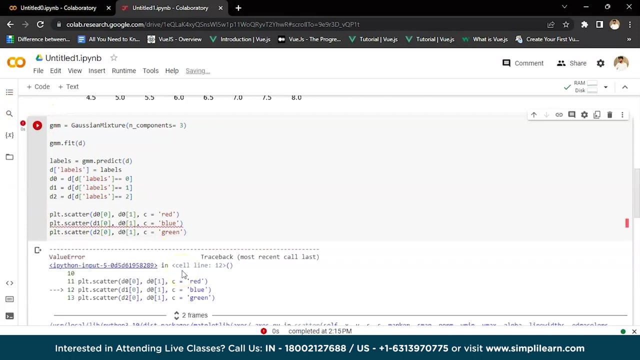 and paste it. one, two and three. okay, so we'll change the value here of d from d1 to d2 and we'll change the color to make it as green. okay, now, as i can see, everything looks good. now we'll execute this code and you. 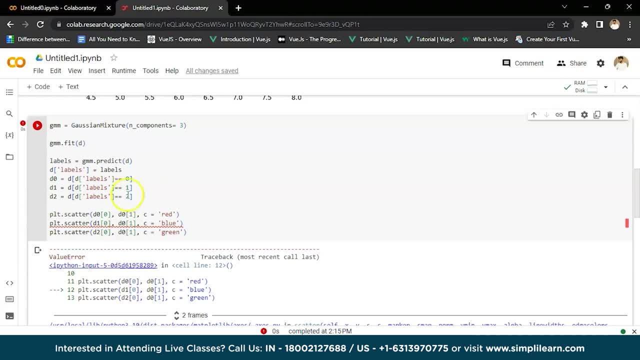 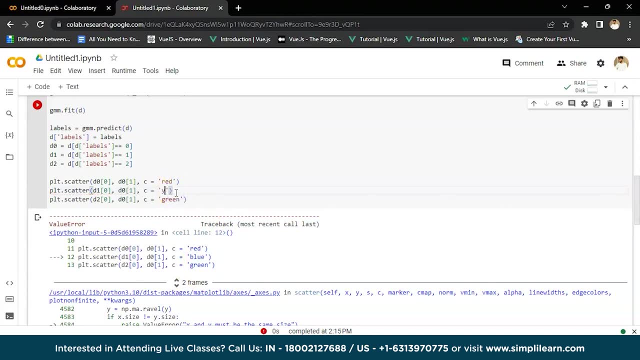 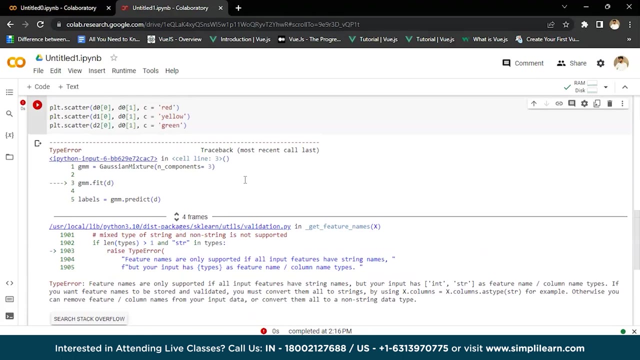 will see. okay, what i have missed here, check again. okay, we have to change the color of this. let's make it as yellow. okay, now let's execute this again, showing us one error for the fit gmm dot red deal. let me check again now. as you can see, 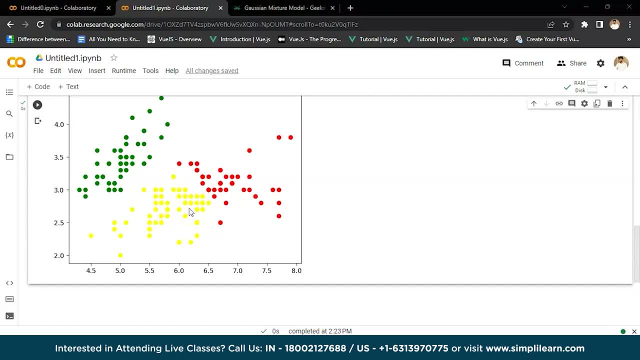 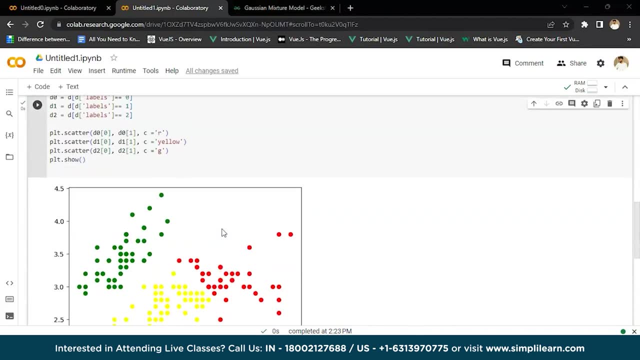 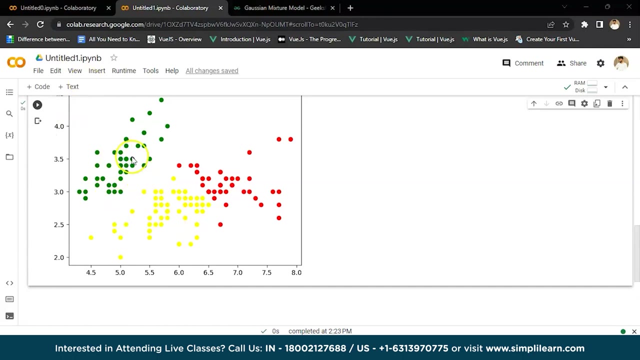 we have the output and in this output you can clearly see that this data, which was previously like this, where we can't see which data is for what, and now, with this gaussian mixture method, we can see all the output in different colors. so we can say that this method helps us very much. 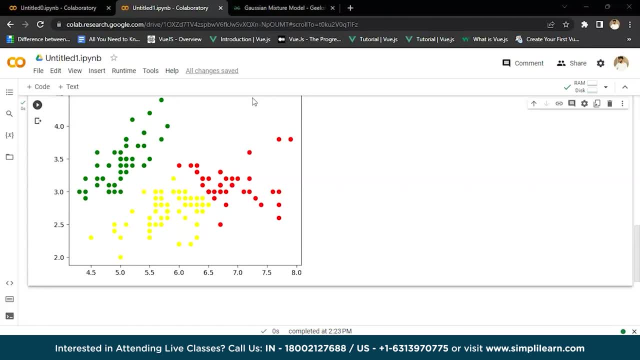 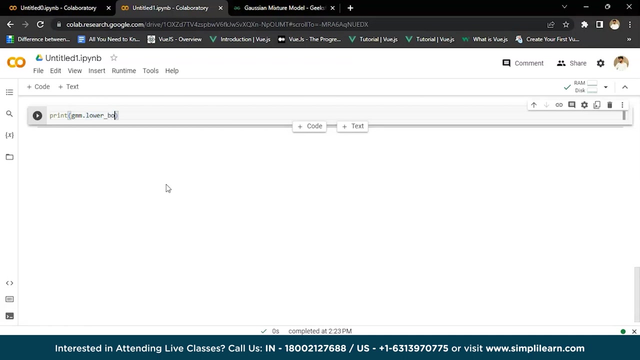 and print the cover log like hood value and number of iteration needed for the model to coverage. okay, so we need to cute a little more code to get the value of that. so for that we'll write print question: mixture model- lower bound, and we will write print gmm, yes, okay, now let's run this and now we have the. 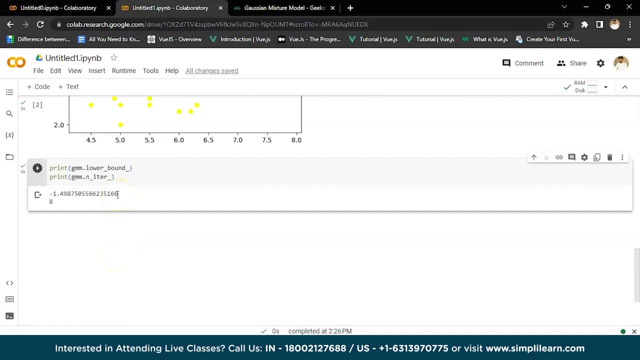 output date and it's the value of that output. okay, hence there are seven iterations for the log, like hood to coverage. so in some reading, garbage is a good example of how the output could be changed, if there are. Gaussian mixture model represents data as a mixture of Gaussian distribution model. 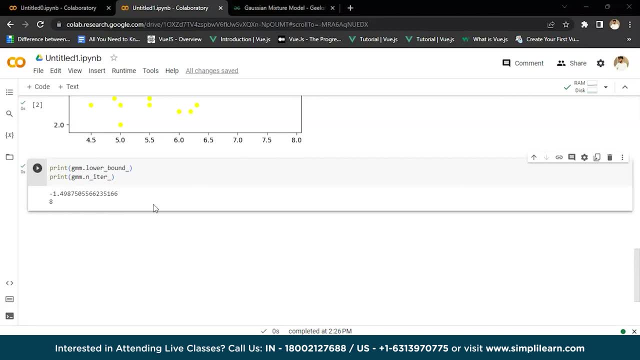 The model's parameters, including the number of components, mean covariance and mixture weight, are estimated using techniques like the expectation maximization algorithm In mixture model. it can be used for clustering data into groups and estimating the probability density function of the data. So with this we have reached the end of this video. 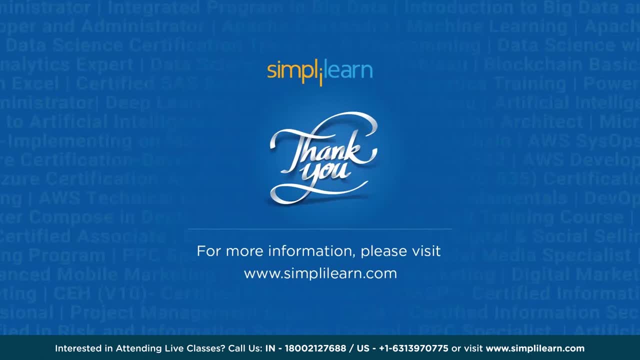 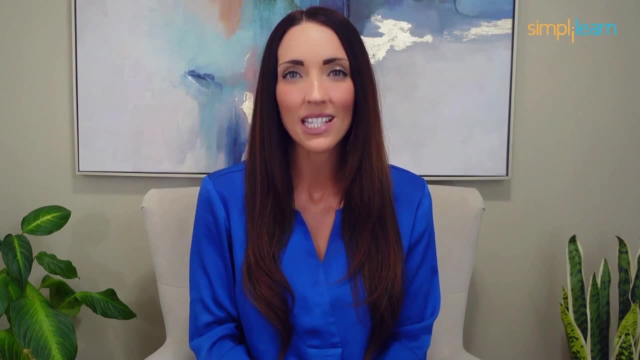 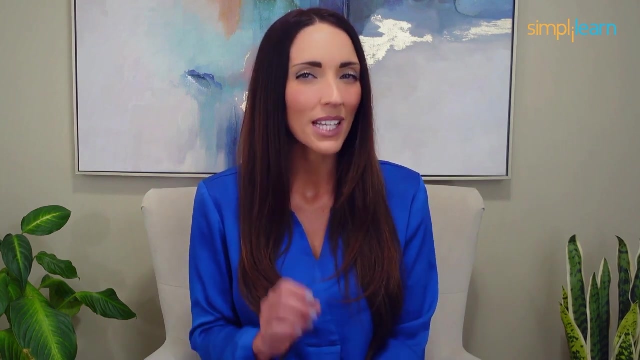 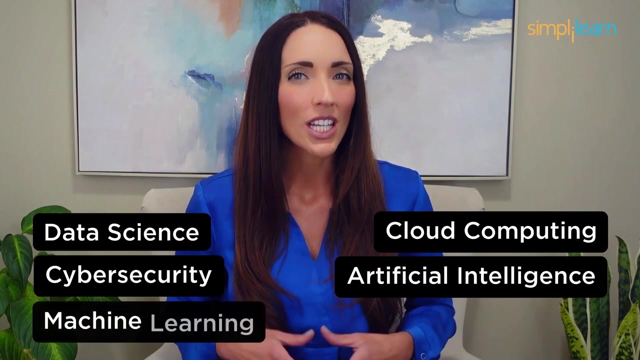 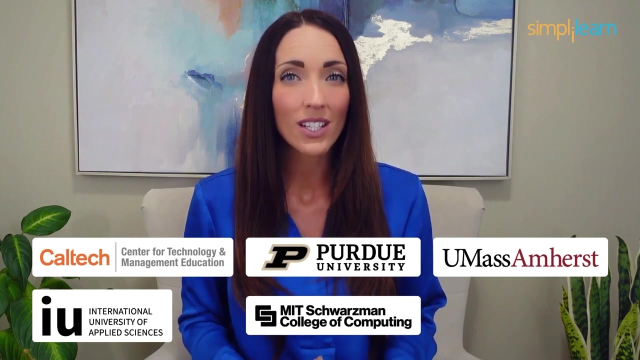 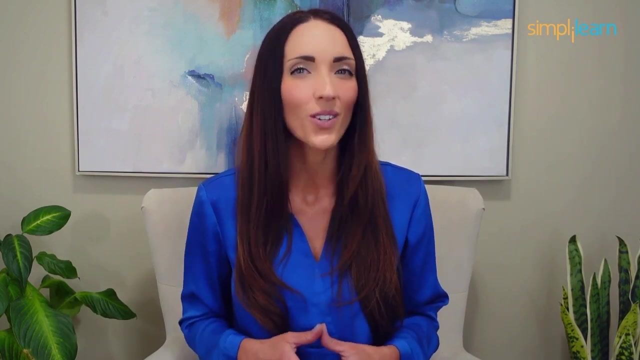 Make sure to like and share this video and subscribe to Simply Learn's YouTube channel. Thank you. AI, machine learning or digital marketing, Designed in collaboration with leading universities and top corporations and delivered by industry experts. Choose any of our programs and set yourself on the path to career success. 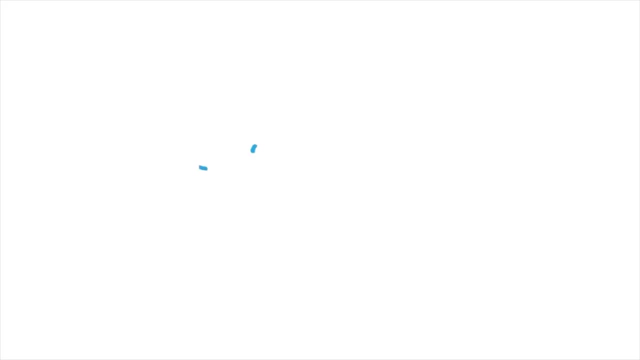 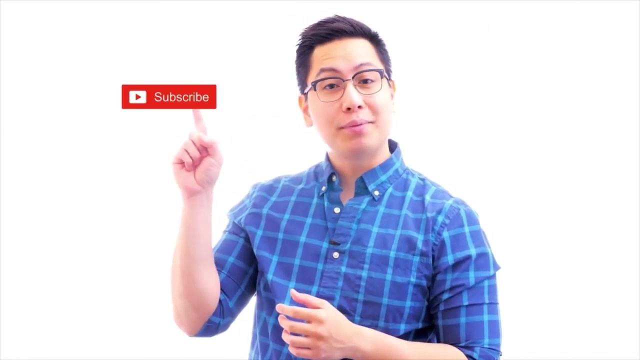 Click the link in the description to know more. Watch similar videos. To nerd up and get certified: click here.